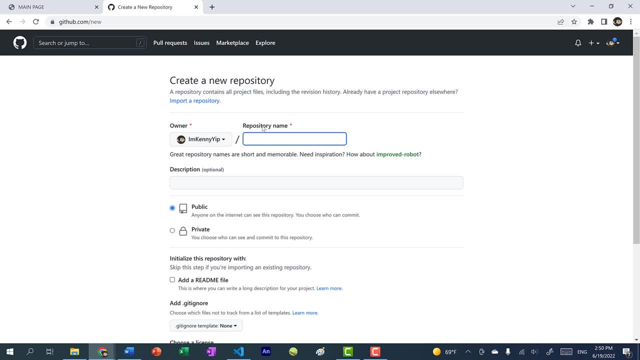 my channel. so if it's a personal website, you want it to be something like your username. so in my case, my username is i'm kennyyip, so you want it to be your usernamegithubio, so you want it to be in this format. so, on github, this will be your landing page for your personal website. now, if you, 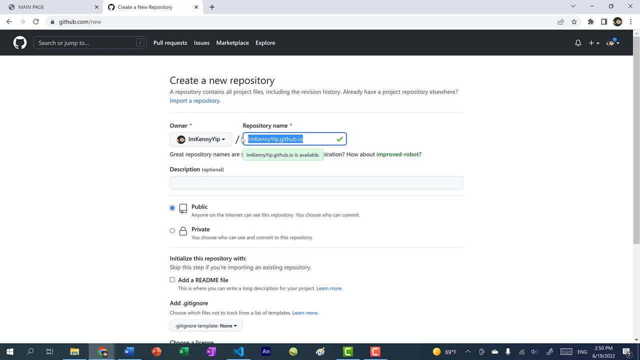 are not uploading a personal website, you can name it whatever you want. so in this case, because it is my personal website, i'm going to leave it as that. but if you are uploading a game or a web project that is not your personal website, you can name it something else. so let's say, if i made a 2048 clone, i would just name it 2048, like. 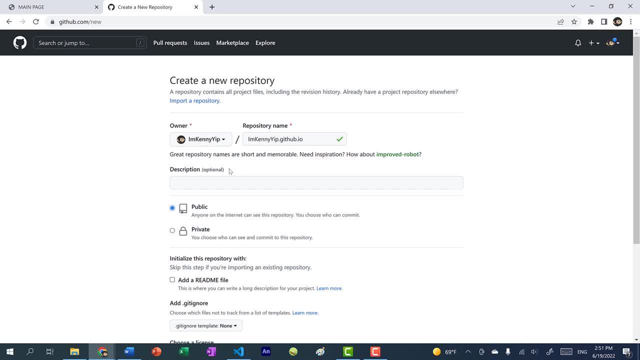 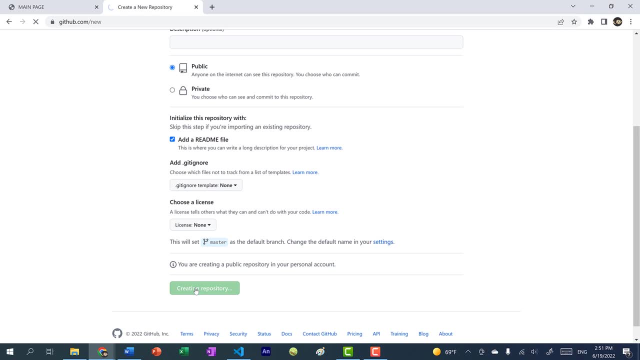 that all right. so i'm going to leave it as that, and then you can leave everything else blank. you can add a readme if you want, it doesn't really matter- and then we're going to click create repository. all right, so from here, if you have git, 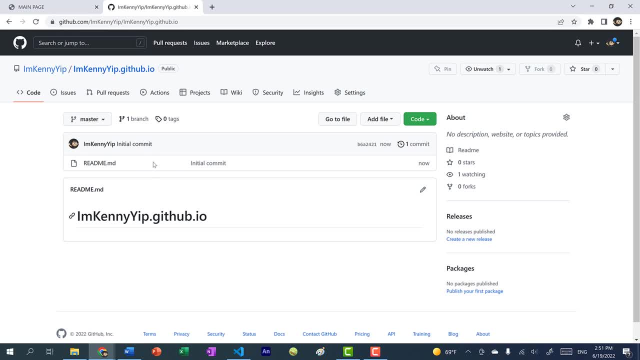 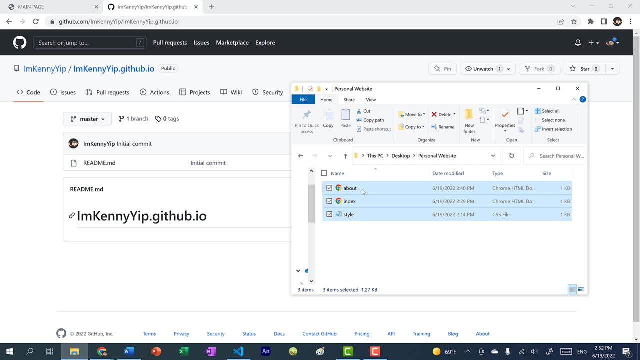 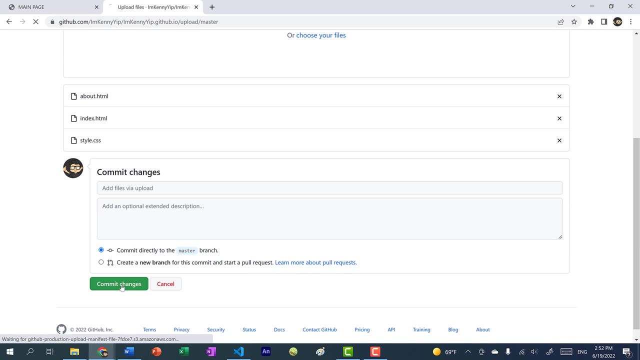 you can use git to push your code into this repository, or you can just open up your folder and highlight your files and just upload via drag and drop. so that's what i'm going to do here, And then again just make sure you have your indexhtml and I'm going to click commit changes. 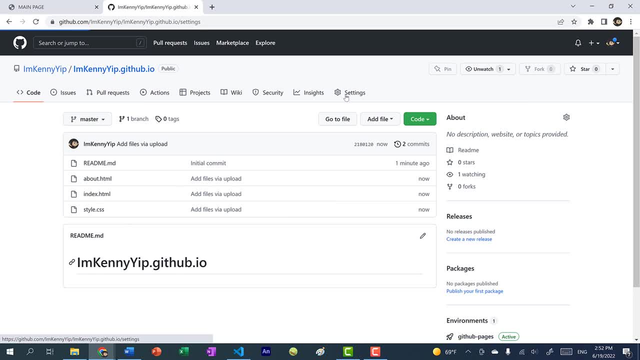 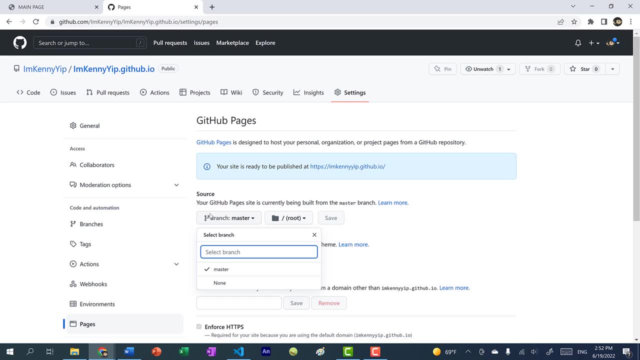 So after you've uploaded your files, just go to settings over here, go to pages and then you want to select source. so i guess here my site is already ready, but yours would probably say none. so click on source over here. click your branch, it'll probably be master or main. click that one. 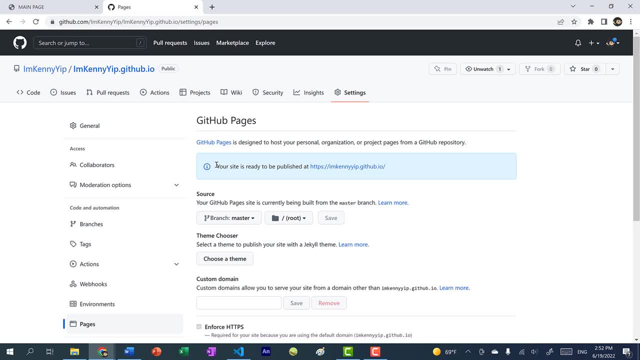 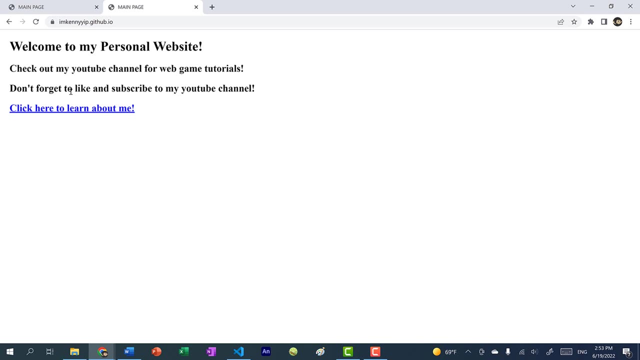 and then click save and then you can see. you'll see this pop-up. your site is ready to be published, that i'm kennygithubio for me, or in your case it'll be your usernamegithubio. so if you click on this, you can see i have my web page already hosted. and to show you a website that is not my: 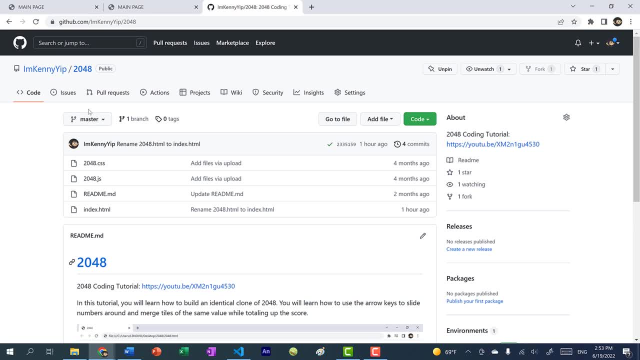 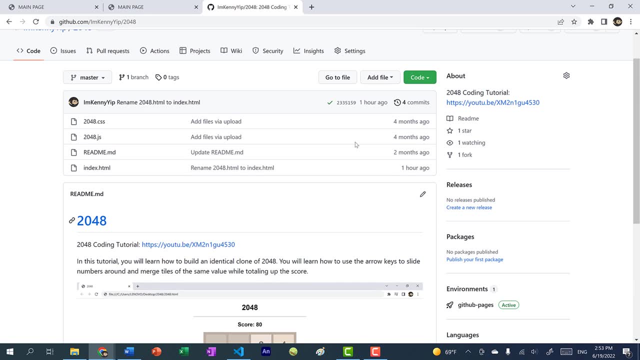 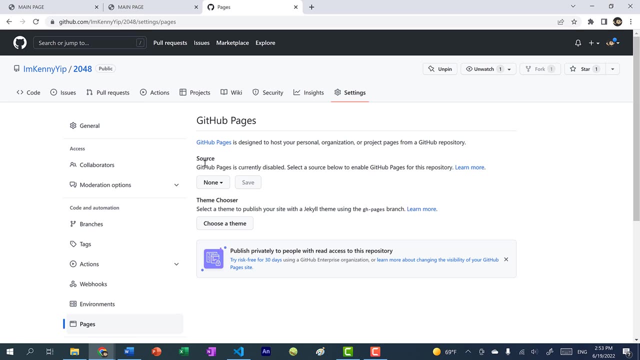 personal website, so it uses a different repository name. for instance, this game of 2048 that i made. i also have a tutorial on that on my youtube channel, so feel free to check it out. i just need to do the same thing: go to settings, click on pages and in here, source, i click on this. 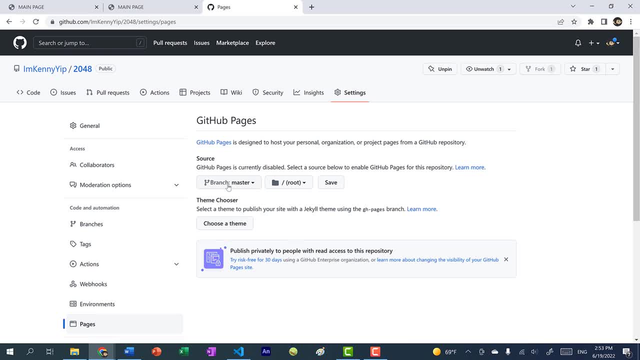 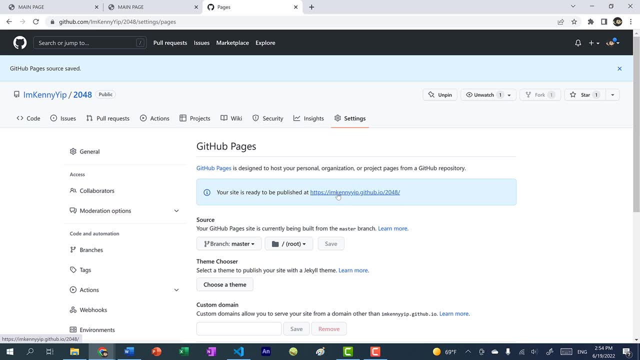 master branch or main branch, depending on what yours says, and i click save and then you can see the link is a bit different in that it shows my usernamegithubio repository name. okay, so that's just the difference between the two: your personal website and which would be your landing page, and 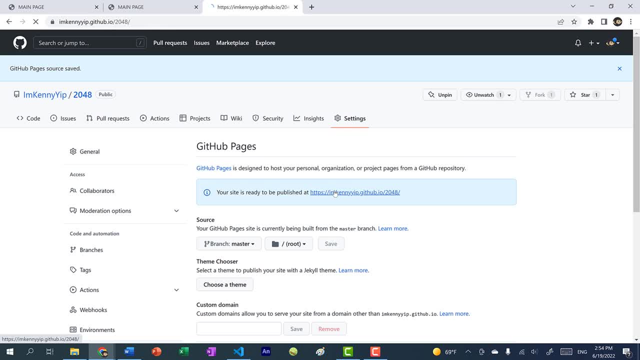 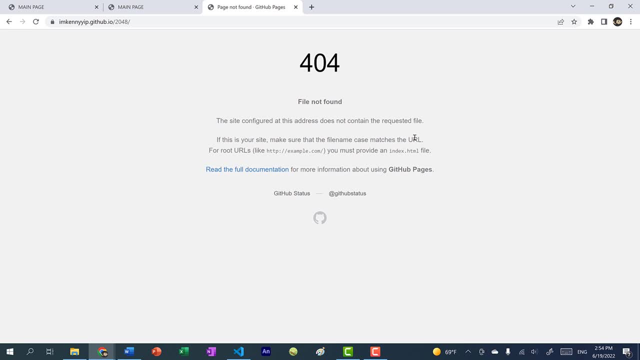 your other project websites. so you can see here it hasn't uploaded yet, but don't panic, you just need to wait like a minute or two and it will show up, and here we have it. we have the 2048 game uploaded and of course i can play it, and yeah, so that's how you upload your website onto github. 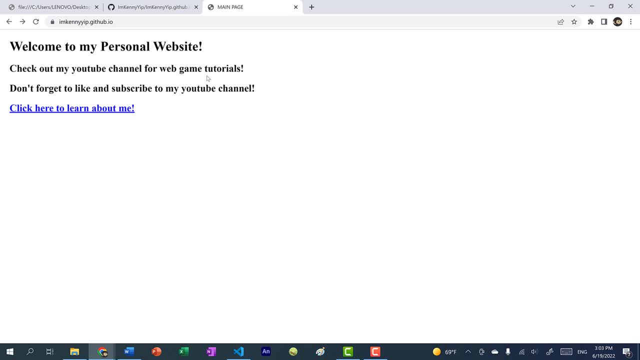 pages. so here you can see i have my personal website hosted. uh, just one more thing, and that is: if i click on this link, it'll take me to the about page and you can see we have about the html, and if i click on the link, back. 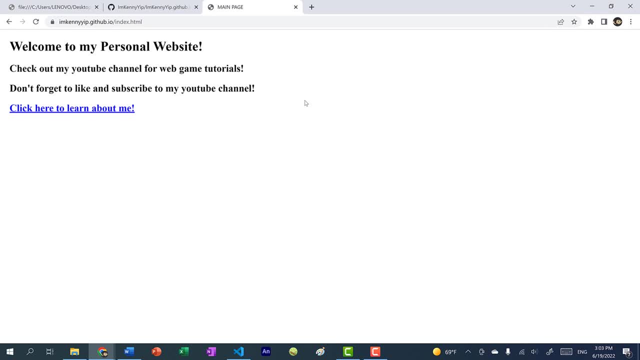 it will give me indexhtml. so this doesn't really affect functionality, but it does look a bit unprofessional and a bit ugly. so we can do something to remove the file extension from our url links. so to do that, just go to your source code, and here we have a link to. about the html. 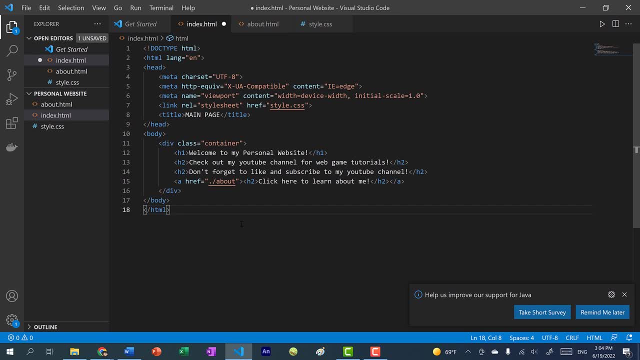 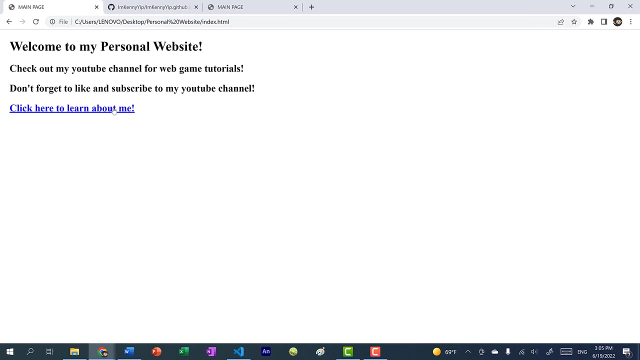 just remove the extension. so we're going to do dot slash about just remove the dot html, and here we are going to remove indexhtml, because indexhtml is the landing page. you do not need the whole thing, you just need the slash. okay, all right. so after removing the file extensions, if i open up the files locally and i click on a link, you can. 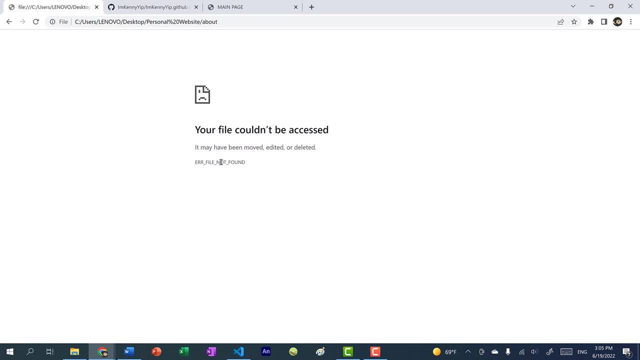 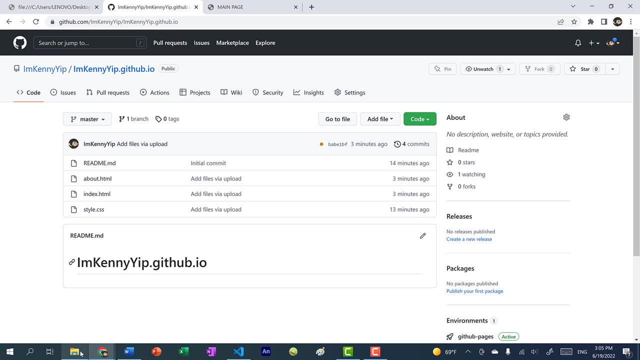 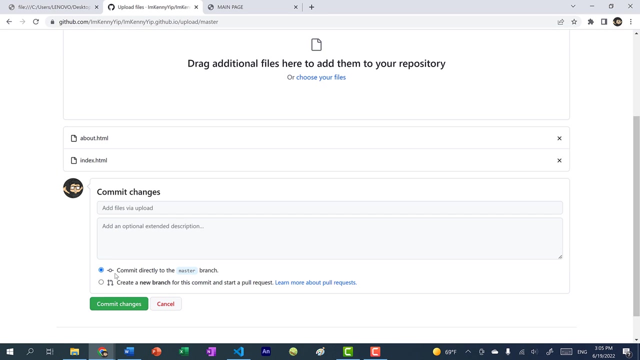 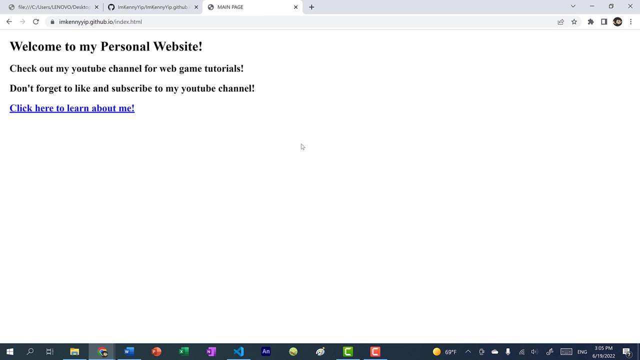 see i get an error. so this error only happens locally. but on github pages it will automatically convert your about to about the html. so all you need to do is just drag and drop your changes, or you can use git and then commit your changes and then give it like a minute or two and it will update. all right, so it's been about a few minutes.